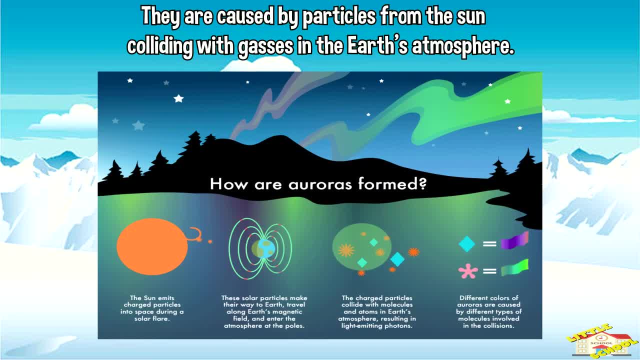 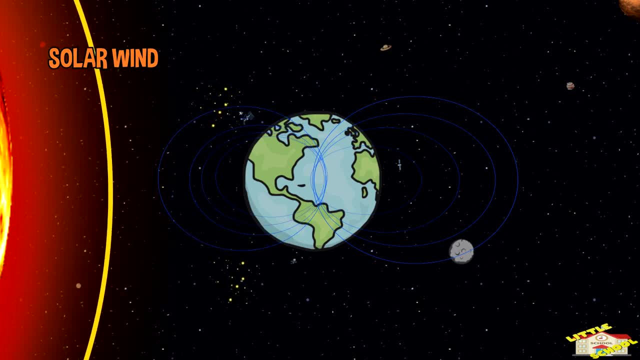 particles from the sun colliding with gases in the Earth's atmosphere. These particles are carried by the solar wind, which is a stream of electrically charged particles that come from the sun. An invisible shield, which is the Earth's magnetic field, will deflect. 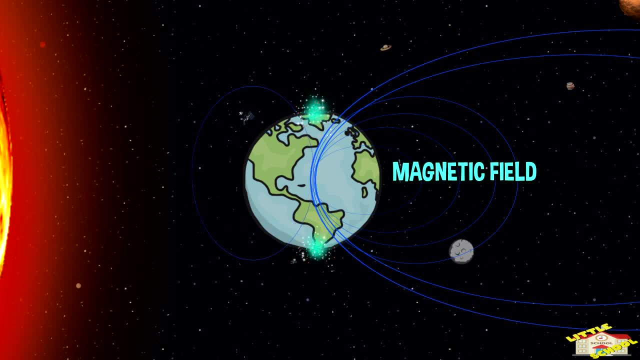 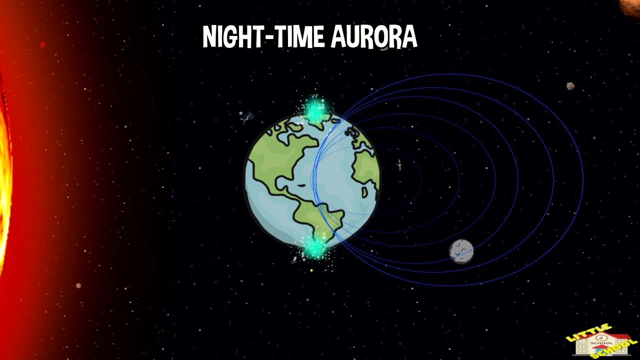 the solar wind Together, magnetic fields will create a funnel for the particles to stream on the daylight side. This is the daylight aurora. The magnetic fields then stretch back and then it breaks, bringing the gas from the solar wind to the night side. This is the nighttime aurora. 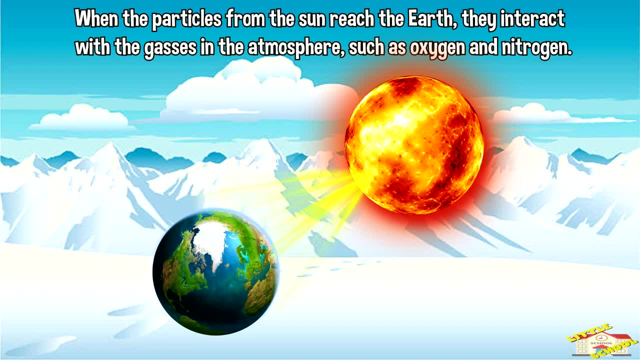 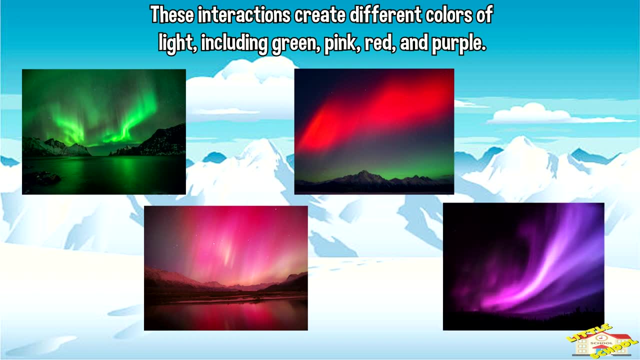 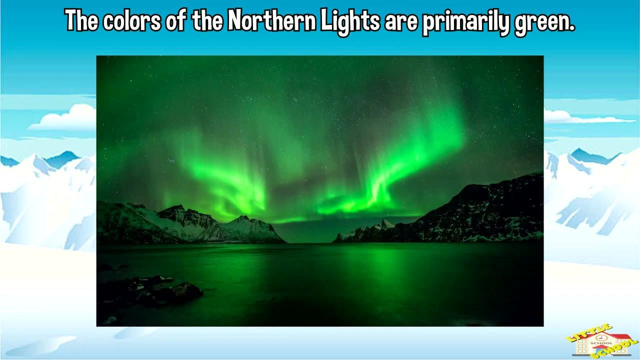 When the particles from the sun reach the Earth, they interact with the gases in the atmosphere, such as oxygen and nitrogen. These interactions create different colors of light, including green, pink, red and blue. High Ž. The colors of the northern lights are primarily green. Green is the most common color and 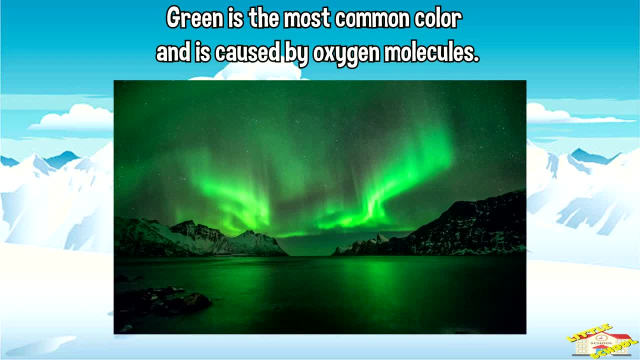 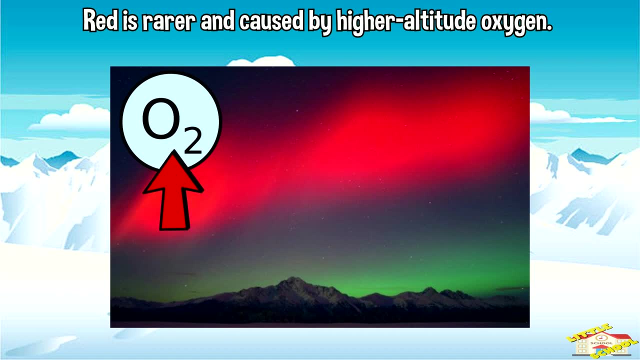 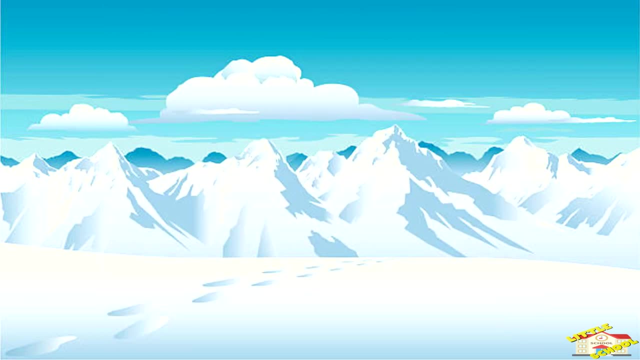 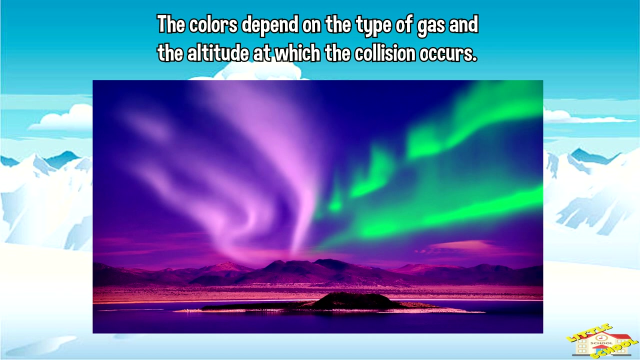 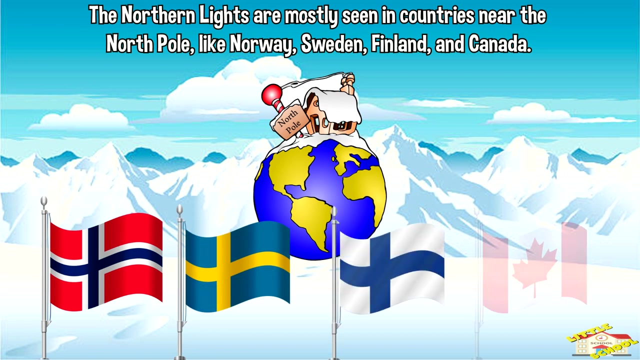 is caused by oxygen molecules. Red is rarer and caused by higher-altitude oxygen. Nitrogen molecules produce purple hues. Low Ž. The colors depend on the type of gas and the altitude at which the collision occurs. The northern lights are mostly seen in countries near the North Pole, like Norway, Sweden, Finland and Canada. 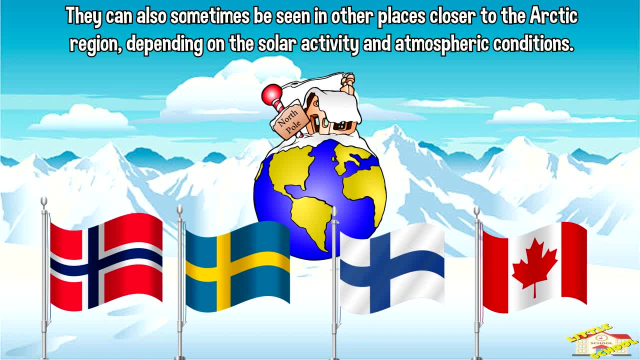 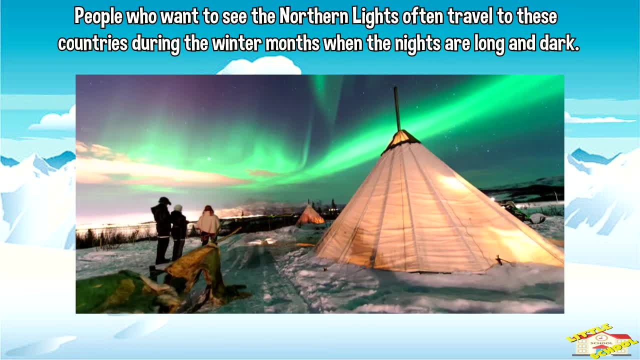 They can also sometimes be seen in other places closer to the Arctic region, depending on the solar activity and atmospheric conditions. People who want to see the northern lights often travel to these countries during the winter months, when the nights are long and dark. The northern lights have been a source of wonder and inspiration for people throughout history. 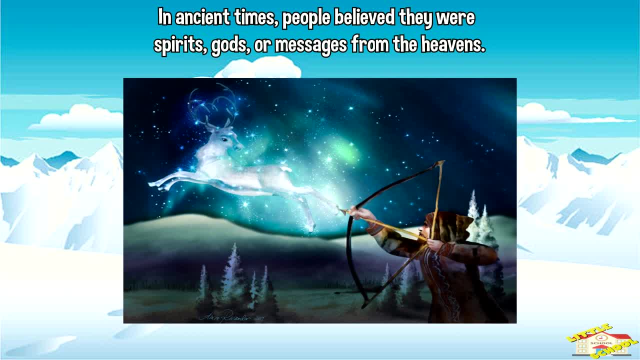 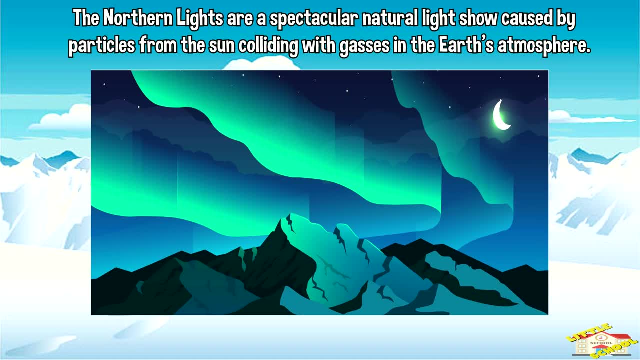 In ancient times, people believed there were spirits, gods or messages from the heavens. In conclusion, the northern lights are a source of wonder and inspiration for people throughout history. The northern lights are a spectacular natural light show caused by particles from the sun colliding with gases in the Earth's atmosphere.